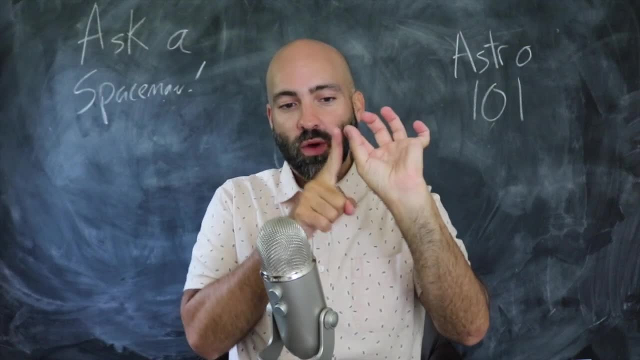 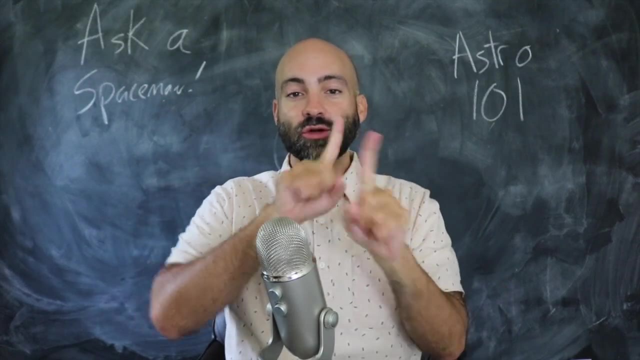 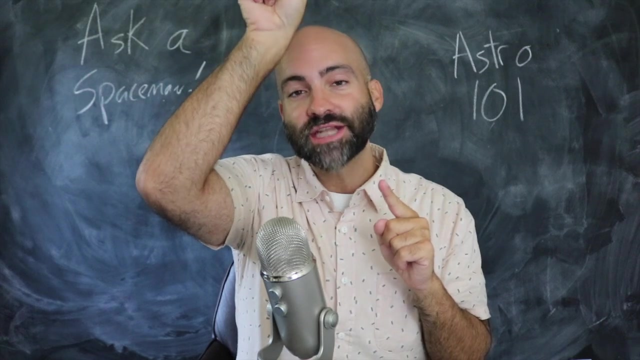 you're going to get. Polaris sits directly above the Earth's North Pole. So if you were to stand on the North Pole of the Earth, of the axis about which the Earth spins, and look directly overhead, Polaris would be at your zenith. it would be directly above you As you go further south on 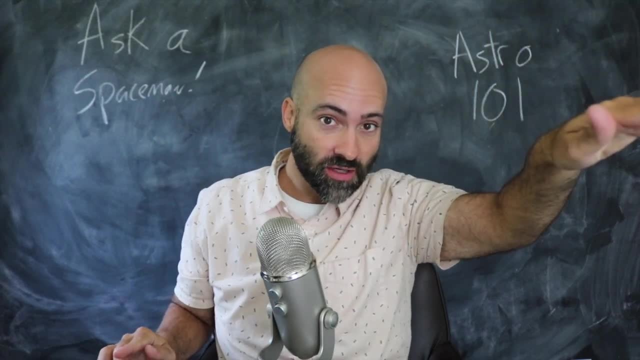 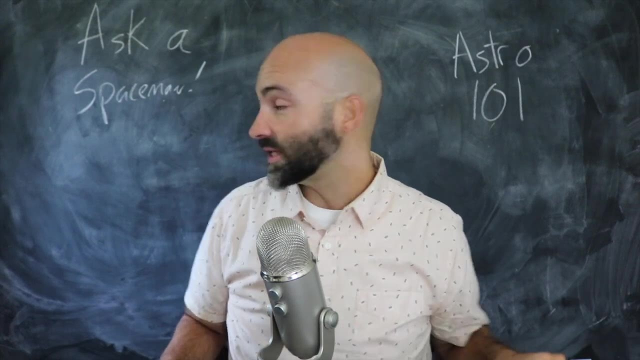 the Earth, Polaris appears to be lower and lower and lower, And if you cross the horizon, then you're going to be at the north pole. So if you were to stand on the north pole of the Earth, then Polaris is under the ground. You can't see Polaris anymore. But then you can turn around. 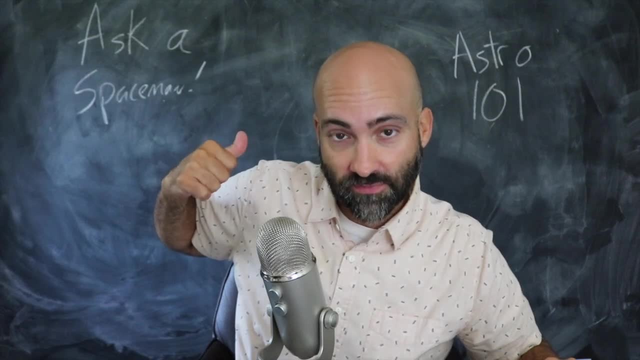 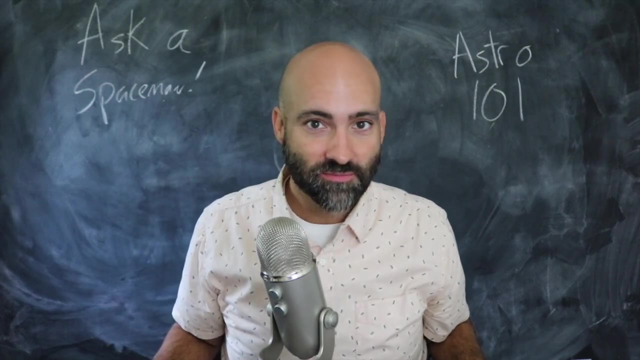 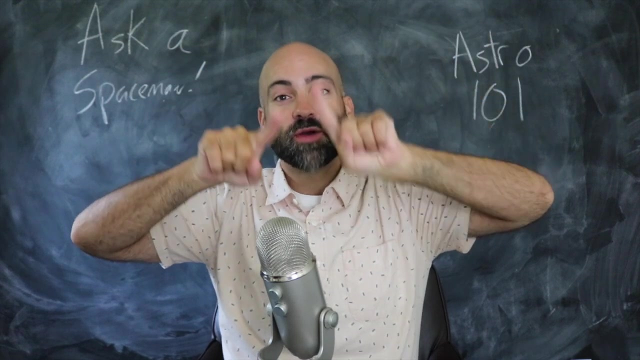 and see the South Celestial Pole. There's another feature that's going to be very important on this celestial sphere, called the celestial equator. So, as you can see, the celestial sphere is like the surface of the Earth, but bigger, and we're on the inside of it. So we have the North Celestial. 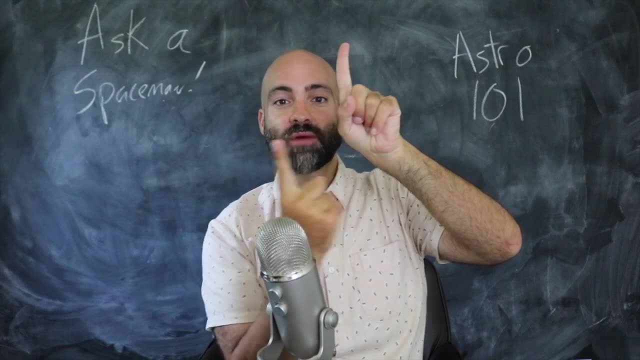 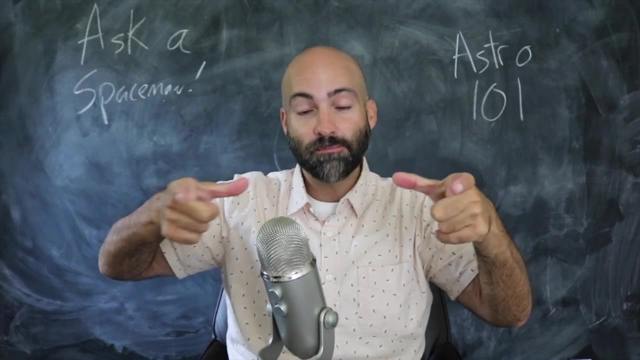 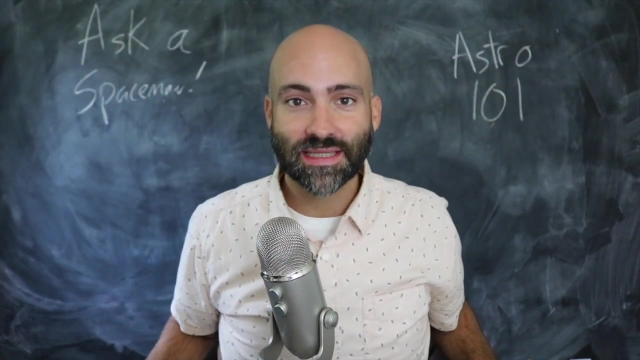 Pole, the South Celestial Pole, and then there's a belt running around halfway between those two poles that we call the celestial equator, just like the Earth's equator makes a belt between our North Pole and our South Pole. Now to identify coordinates on the sky, you know, like on the 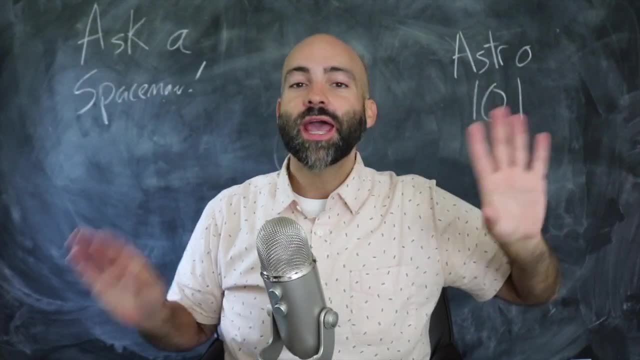 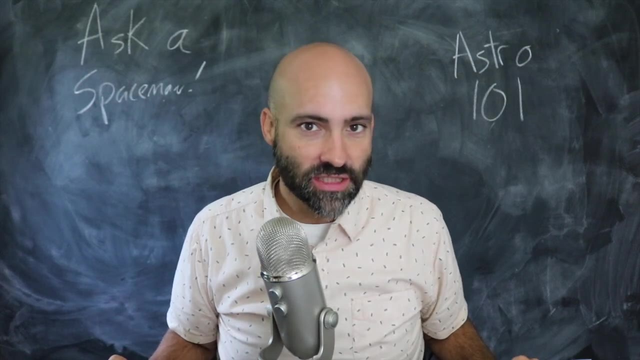 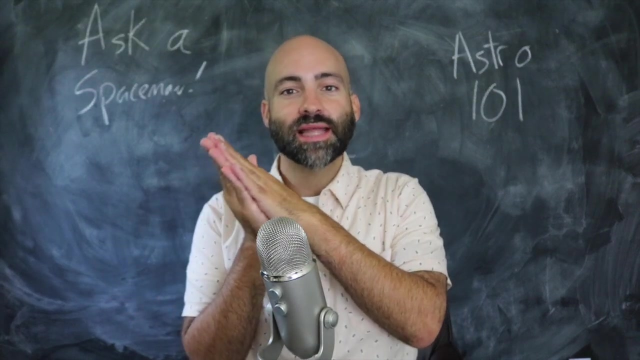 Earth, the surface of the Earth. we have latitude and longitude, We have a coordinate system like that for the night sky. But we call this declination and right ascension. Declination is how far above or below that celestial equator you are. So if you're a star and you're right there at that belt, 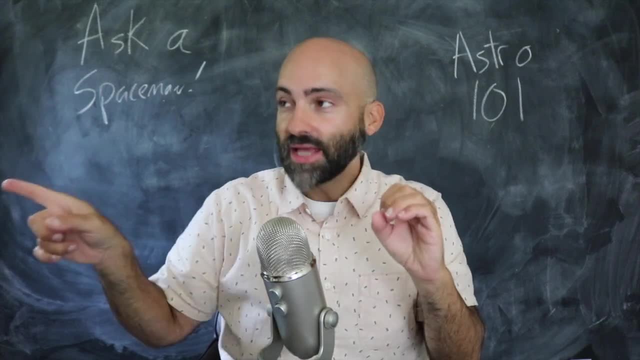 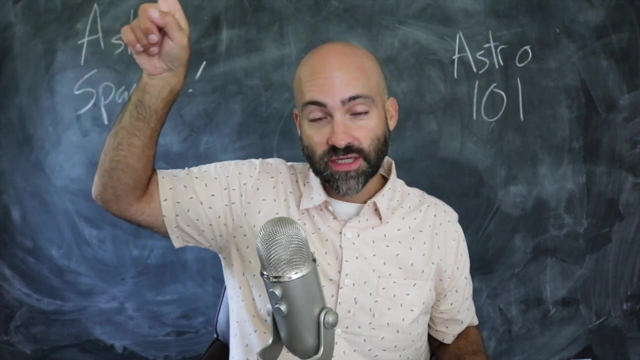 at that celestial equator, you have a declination of zero, And then as you go north from there, you get higher and higher. It's counted in degrees, So you can be like five degrees, 10 degrees, 20 degrees, all the way up to Polaris, which Polaris itself is sitting at 90 degrees. 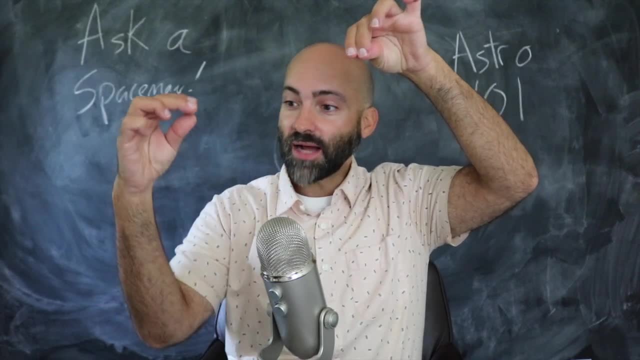 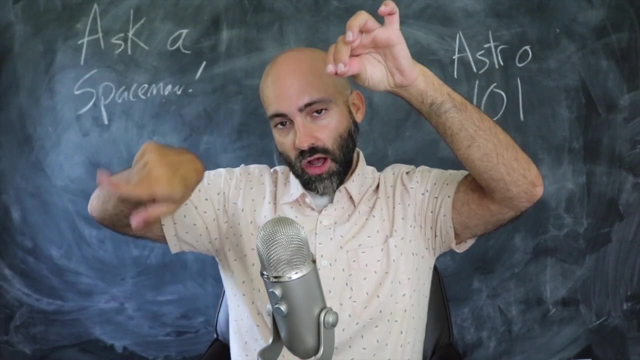 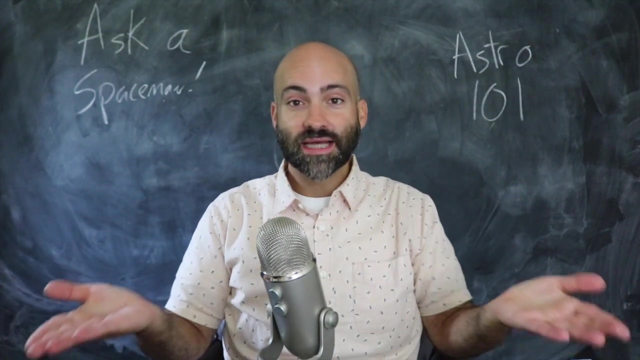 declination, And then for Southern Hemisphere objects or objects below that celestial equator, we have negative degrees like negative five, negative 10, negative 50, all the way down to the South Celestial Pole, which is sitting at negative 90 degrees. So by knowing the declination, you know how far above or below the celestial equator that object is. Now that's the upy downy motion. The lefty righty coordinate is going to be totally arbitrary, Just like longitude on the Earth is totally arbitrary. You need to pick somewhere to be zero longitude and then measure all longitude off of that. 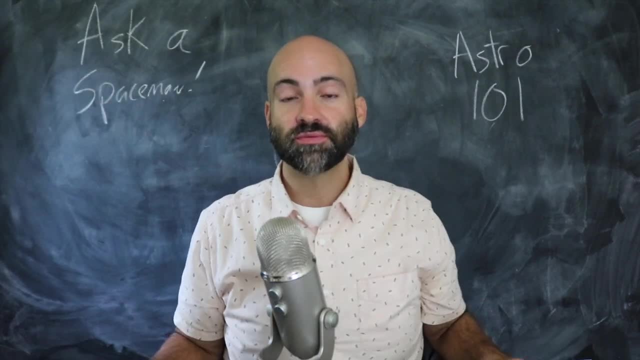 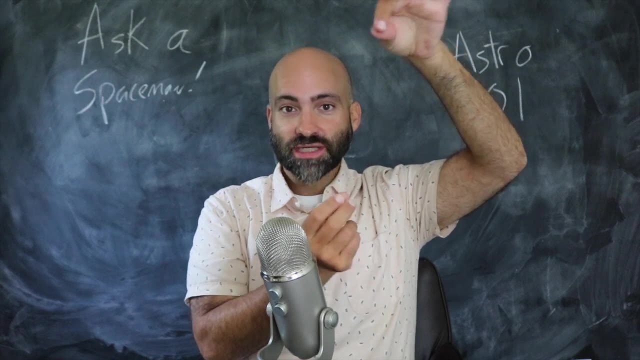 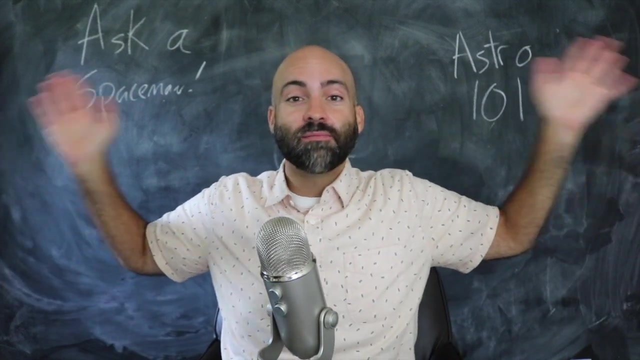 In modern times, we've settled on zero longitude. being the Greenwich Observatory in England, That is the, the line of longitude that marks zero degrees, And then we measure everything off of that. It could have been anywhere. It could have been anywhere, But because of history, it ended up in Greenwich, England, For the night sky that zero longitude- like where are we going to start counting? is going to be where the sun crosses the celestial equator at the spring equinox. Why, Well one, we had to pick something. 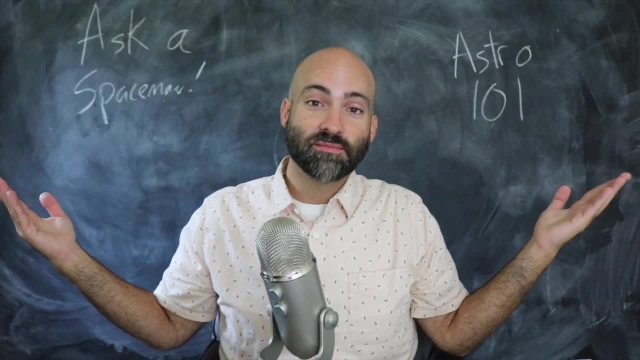 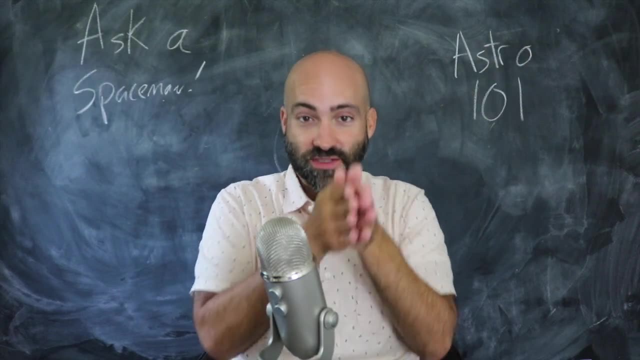 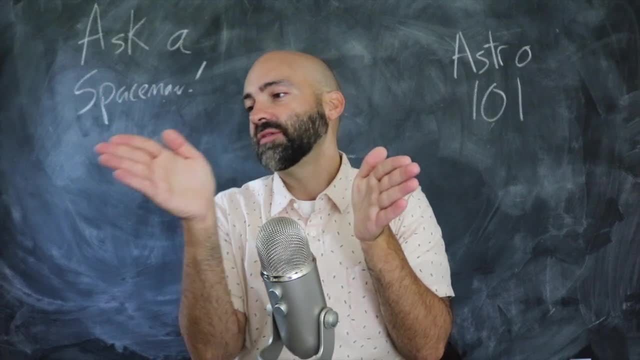 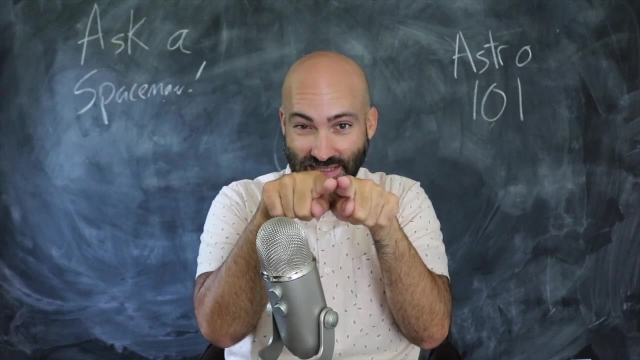 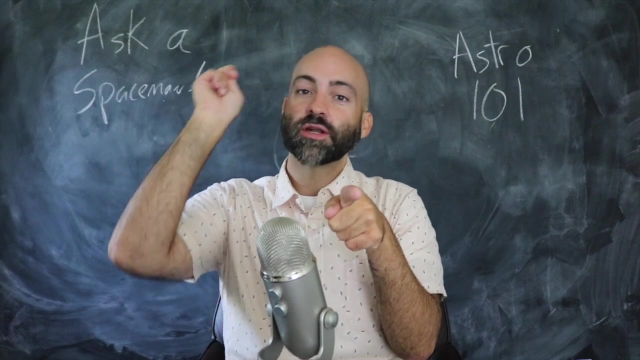 right ascension, And then everything off of that is measured in degrees or, sorry, it's measured in hours, minutes and seconds. So you start here at zero right ascension, And you start making a circle like you can imagine the hands of a big 24 hour clock, So that giant circle going around. 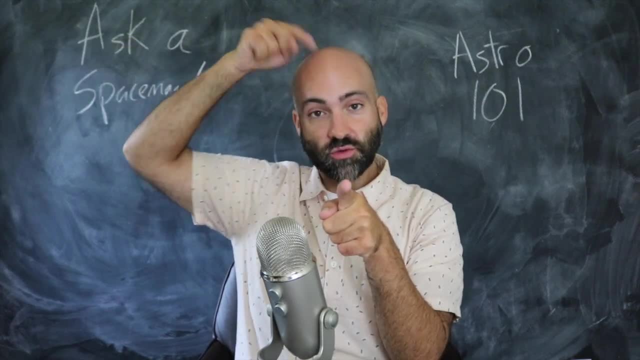 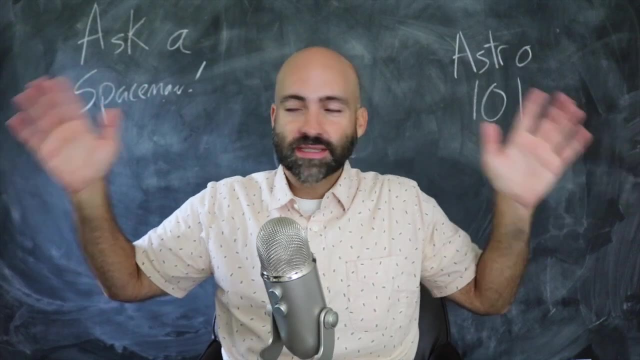 the sky is measured, is cut up into 24 hours, the hours are divided into minutes and the minutes are divided into hours, So that's zero longitude, And so that's zero longitude, And so that's zero seconds. Why? Because reasons, There is an issue here with right ascension and count in depending on the spring equinox. The spring equinox changes where the sun rises, where the sun crosses. that celestial equator changes every year Because the earth itself, our orbits are sorry, our spin, our rotation, we're wobbling a little bit. our North Pole doesn't always point to. 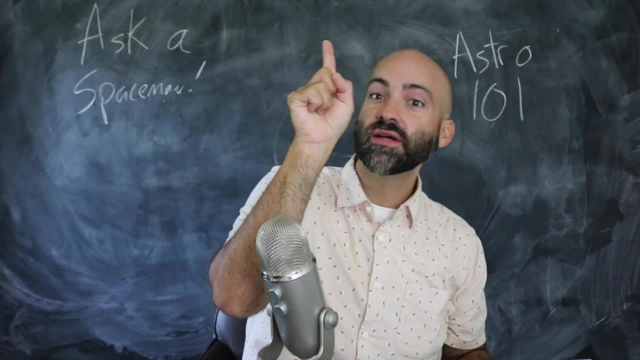 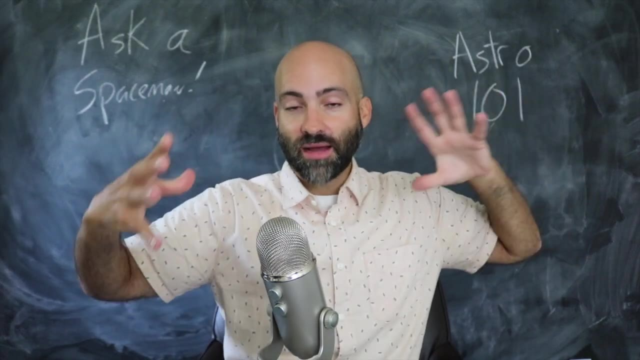 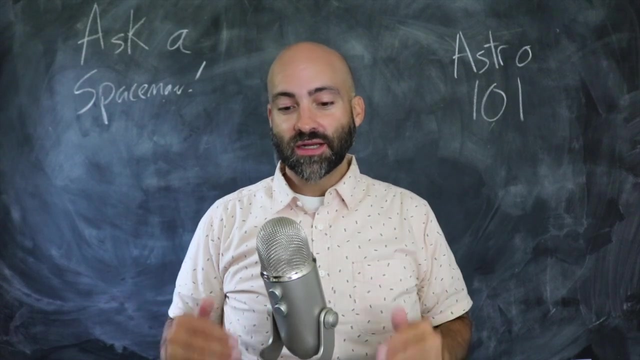 the star Polaris over the course of thousands of years, it makes this tiny little circle in the sky, And so this changes where astronomical objects are according to our particular calendar days. So to account for this, in addition to the right ascension, you basically have to say what. 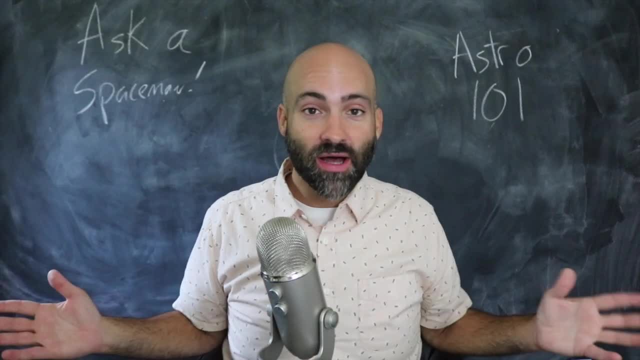 year it is, And in astronomy terms, this is called an epoch, again for reasons, this is all just jargon, So to so to get to the point, we're going to have to say what year it is, And so this is. 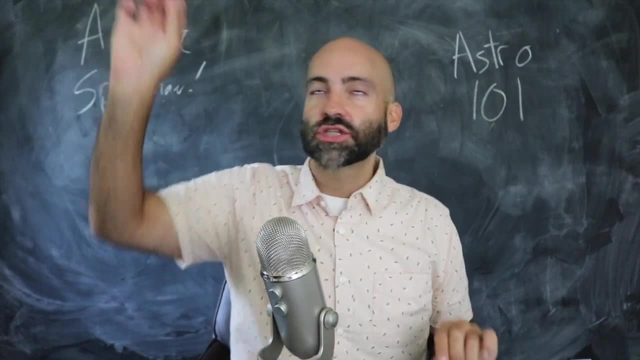 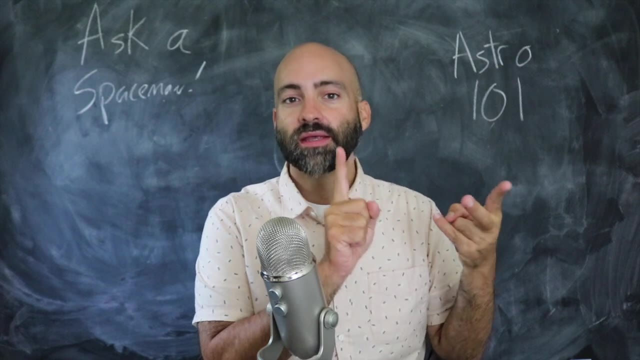 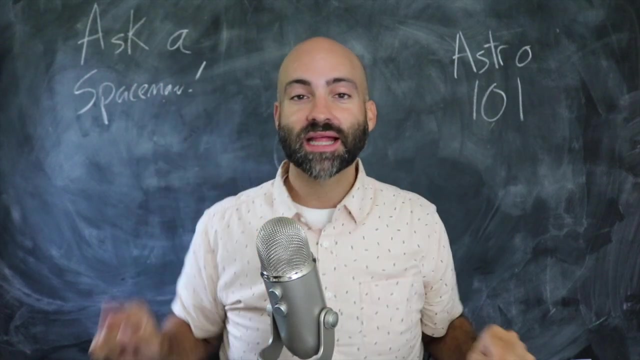 to give a full accounting of exactly where a star or a comet or a planet is on the night sky. you have to give its declination, you have to give its right ascension and you have to give the epoch or year, and that will help pin down exactly where that star is. And it's these. 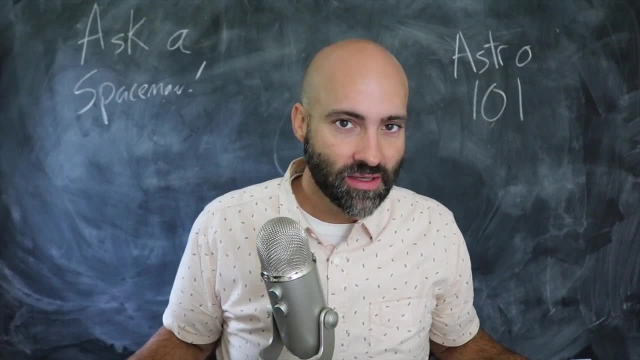 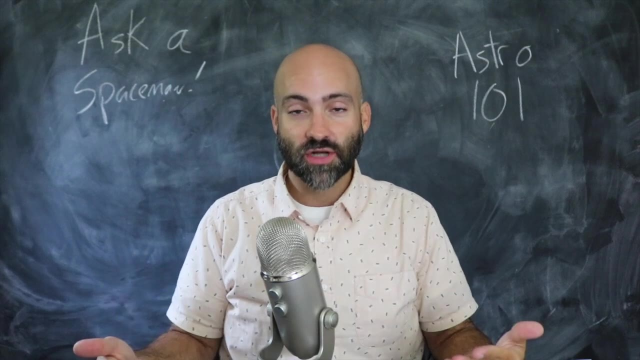 coordinates that astronomers continue to use today. There are a few other things on the night sky, like. there are constellations, there are cool, pretty patterns And, again, because astronomy is based on the Western tradition, we have a lot of Greek constellations, a lot of Arabic. names for stars. a lot of European explorers. So every culture has constellations. About 100 years ago the International Astronomical Union settled on 88 constellations that cover the sky, But you can make up any constellation you want. really, no one owns that, But astronomers use constellations. 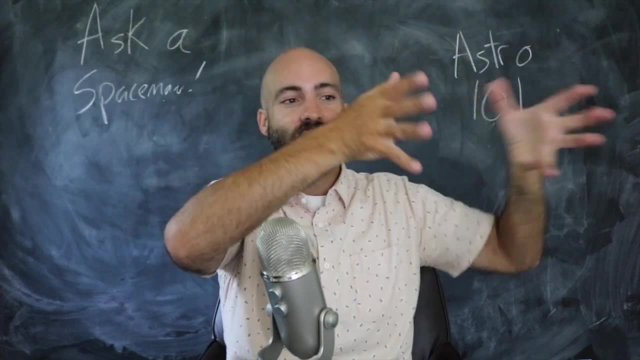 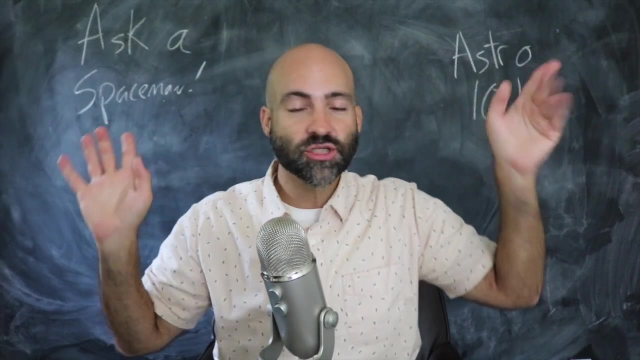 they don't use constellations like for anything other than dividing the sky like, okay, this is in, this is in Capricorn over here and this is in Sagittarius over here. So we know what chunk of the sky a particular object is in. 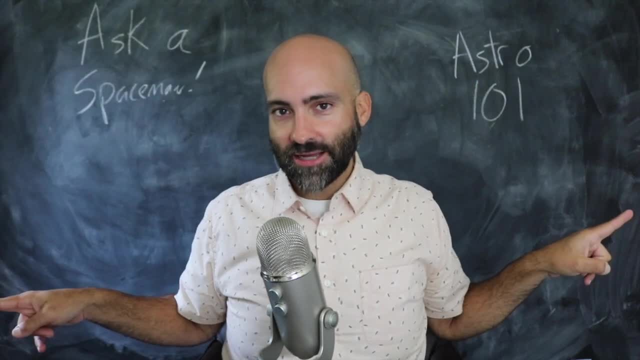 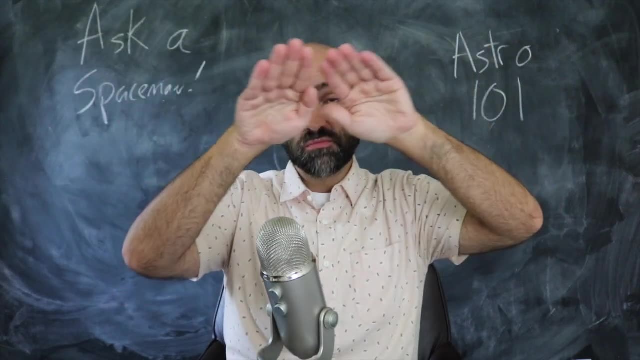 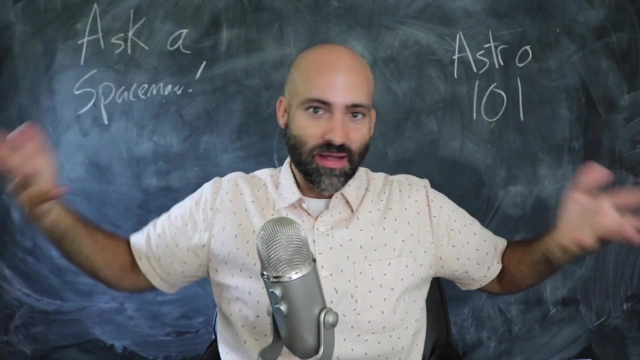 There is a special set of constellations on the sky where all the planets in the sun and the moon appear to move through. Now we know that this is the plane of the solar system, but again, back then we didn't know. we just saw the planets like following particular paths. 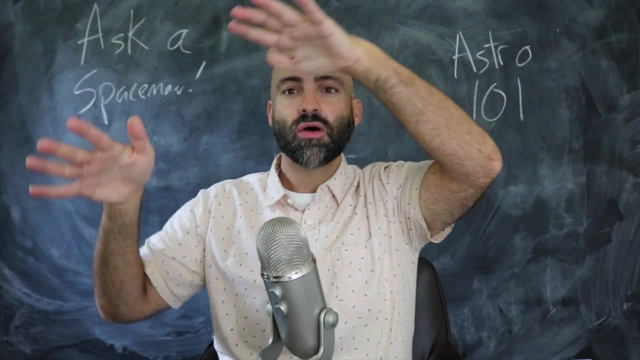 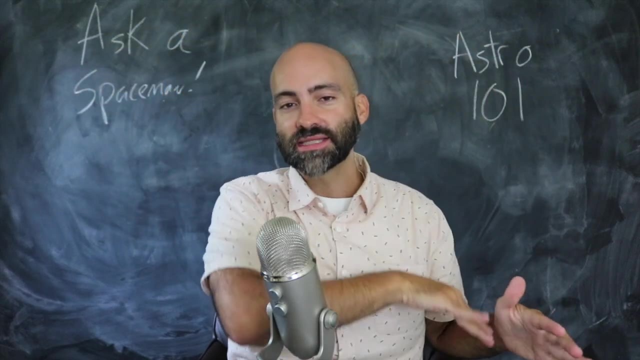 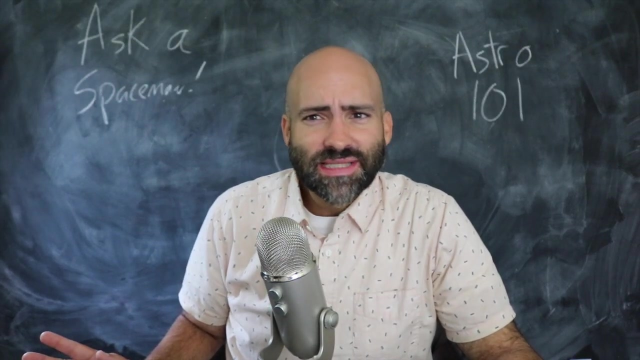 we saw the sun follow a particular path in the sky, And so all these very important things like planets and suns and moons are moving through a distinct set of constellations. we call that the zodiac. There are actually other constellations that the sun moves through but didn't include. get included in the zodiac because reason People care a lot about the zodiac because of you know horoscopes and predicting your future, which was a huge deal back then back in the day hundreds of years ago, is not so much a huge deal. 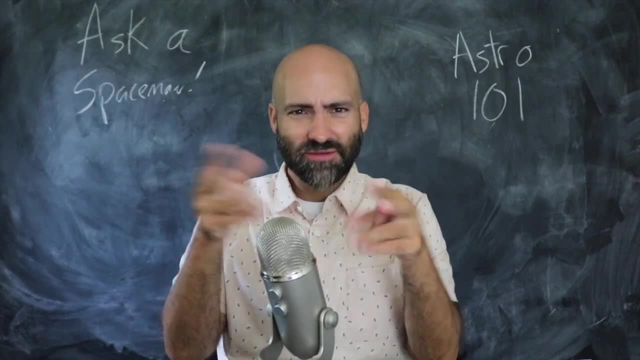 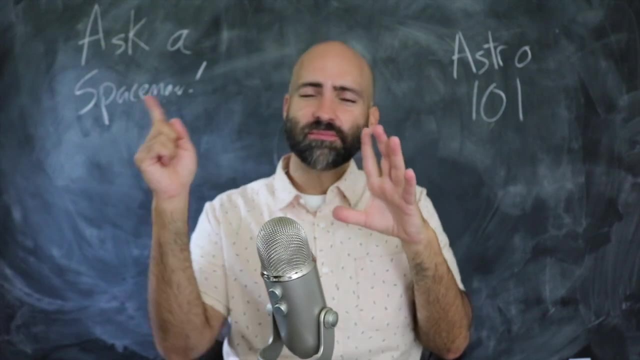 now And, in fact, your sign, if you know your, your sign, like what month you were born in or whatever. it's actually wrong, actually, because of that procession of the of the earth, of our axis. it's been a enough century. By now that your sign that the constellation that you think you were born under is actually one over. just thought you would know. no, it has no connection of what- where the sun is, where the planets are in in the sky, has absolutely no connection to your everyday life. Because stuff? 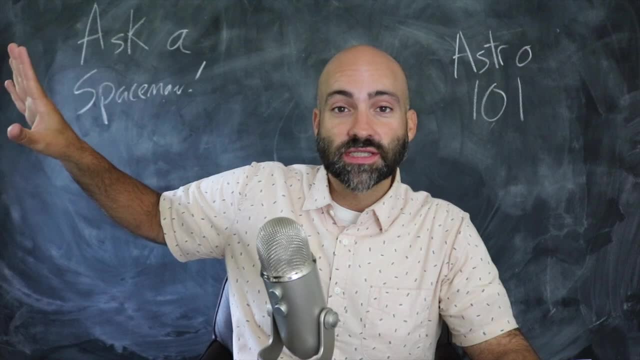 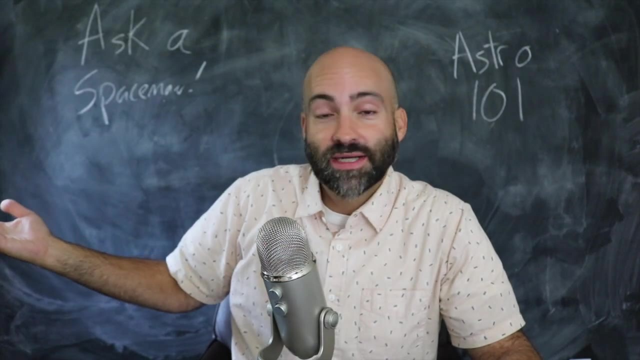 in space is really really far away And we understand the forces of nature And like it's you can see them in their pretty- which affects your life. I guess, like if you're going to go out on a nice beautiful evening and stargaze and look at the planets, that that can change. 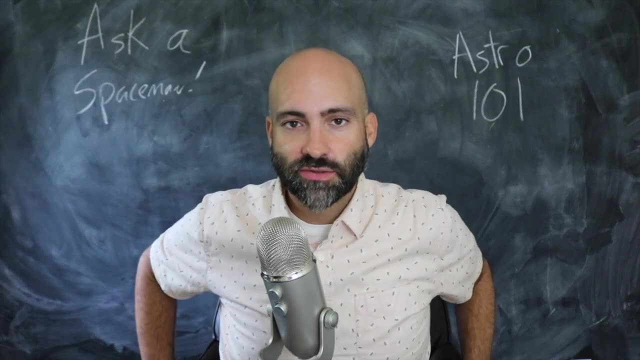 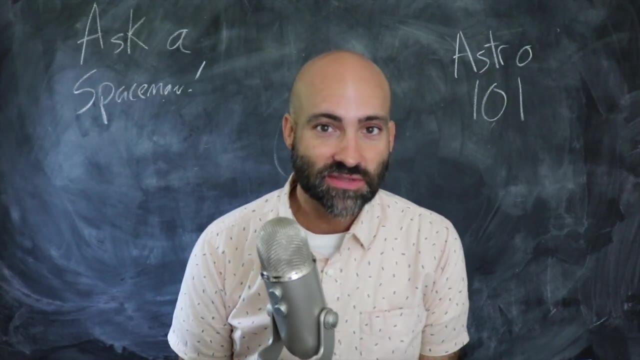 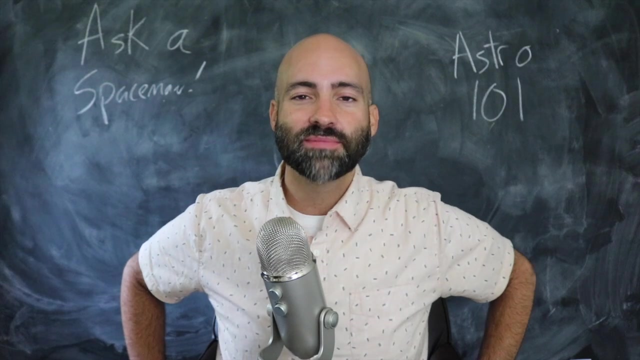 your life, but not in any real like direct way. So that's the night sky. we're gonna keep going with this Astro 101 series coming up. Next we're going to look at the solar system. So tune in. then don't forget to go to patreoncom slash PM Sutter to help support.